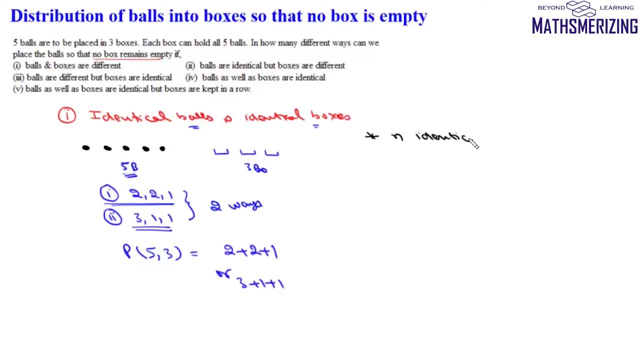 balls and r identical balls boxes, then this number is same as partition of number n in R. So we have to find total number of ways in which we can partition a number n in R compartments. Now when n is large it is very difficult to find this P. 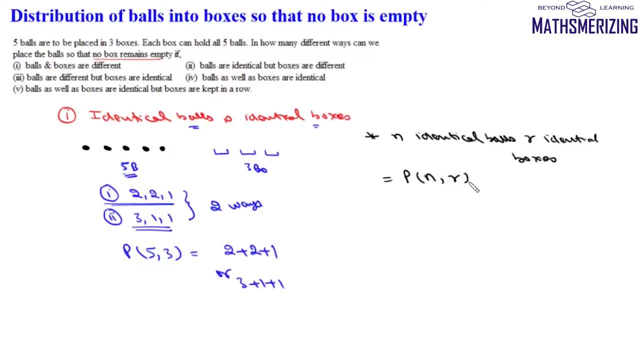 Suppose we say we need to find number of ways of distributing nine identical balls in three identical boxes. So in that case this n is nine. Now, how do we solve such cases? So for that we have one theorem, and that theorem it might come to our rescue. and the theorem 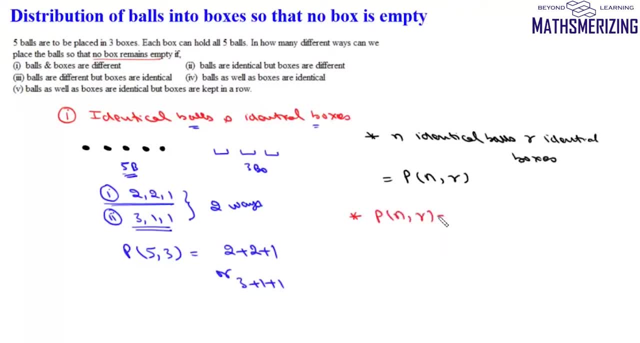 is. we can write this P as the summation P, where k varies from 1 to R. So say, for example: suppose we have a question where we have nine identical balls- Okay- And three identical boxes. we need to find number of ways in which we can distribute. 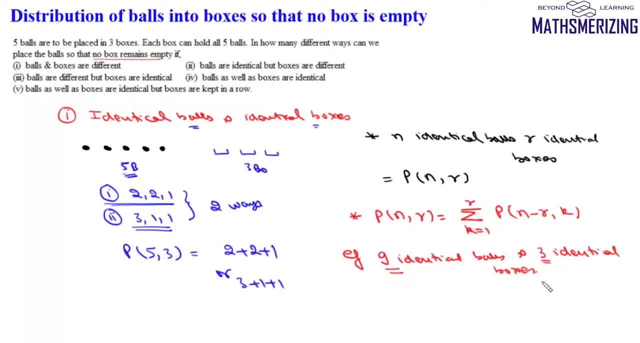 nine identical balls in three identical boxes, so that no box is empty. So we know that it is given by this partition P. We can write this as summation: P Now, n minus R. n minus R in this case is six and six comma. 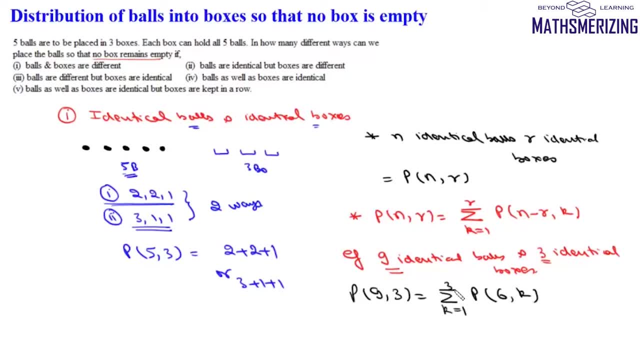 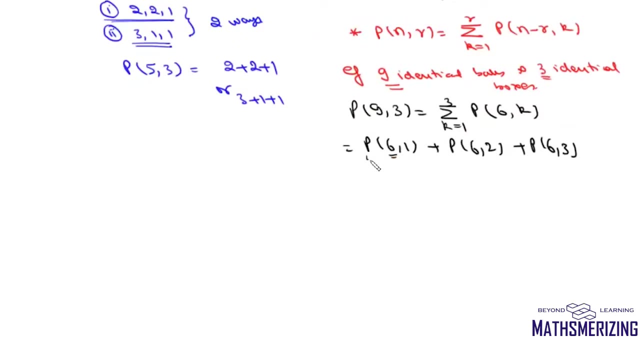 k, where k varies from one to three. So it will be P plus P and P. So this problem now reduces to partition of six in one. So in how many ways we can partition six in one part? So we know that we can do it only in one way. 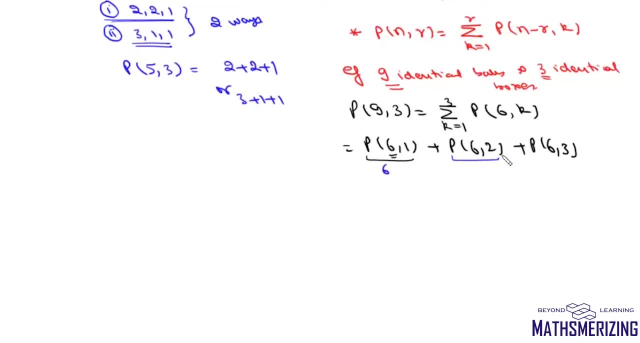 So it will be simply six. What about six in two? Six in two is either five plus one, So we know that we can do it only in one way, So it will be simply six. What about six in two? Six in two is either five plus one, or four plus two, or three plus three. 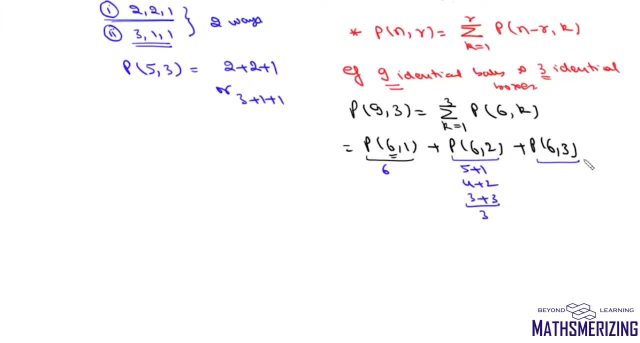 So there will be three ways. And what about six in three? Six in three will be either four plus one plus one, or three plus two plus one, or two plus two plus one, which again is three. So it will be one plus three plus three. 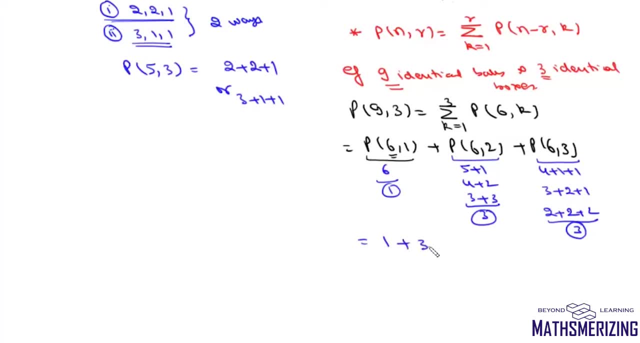 So P it is one, P is three And P is three. So this result: it comes out to be seven. So the number of ways of distributing nine identical balls in six identical boxes is seven. So any such problem we have to solve using partitions. 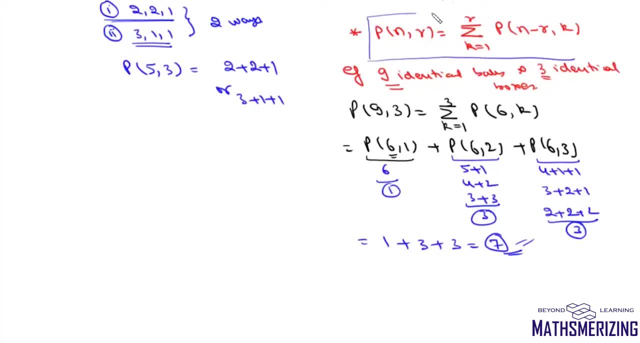 And there this theorem will come handy if the value of n is large. And this is how we solve such problems. Now, if the problem is not asked in an examination and we need to find partition of n into r, then we can also use this partition chart. 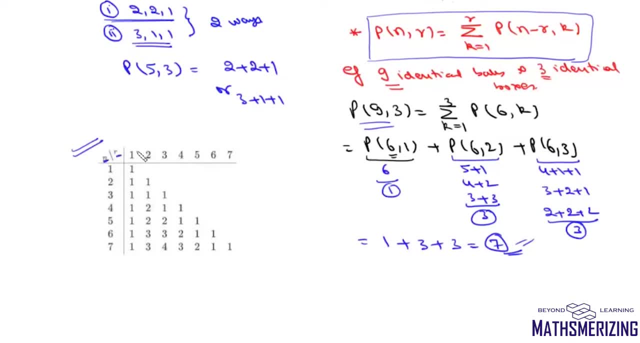 Okay, So here we are, given n and r. Then, using this table, we can clearly find out the value of P and r. Suppose we need to find the value of P, So P it will be one, So we have this value one. 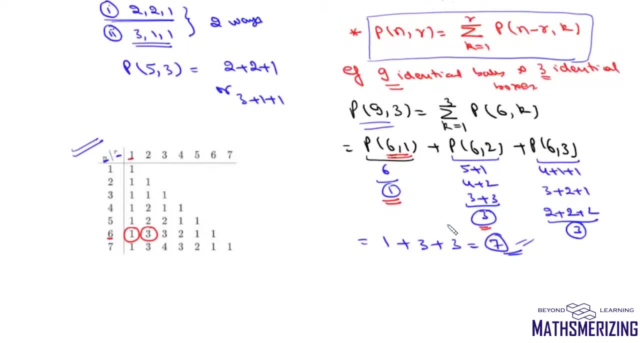 And then P. P is three, We have got the value three. And then P is again three, So it will be again three. So it will be one plus three plus three, And that again is seven. So this is how we solve problems: when the balls are identical and the boxes are also identical. 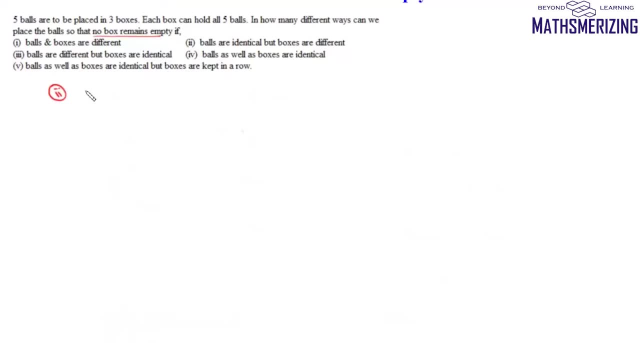 Okay. So the first problem is is that the number of balls on the left side of the table is identical. The number of balls on the right side of the table is also identical. Now we will come to the second case, when balls are identical and boxes are distinct. 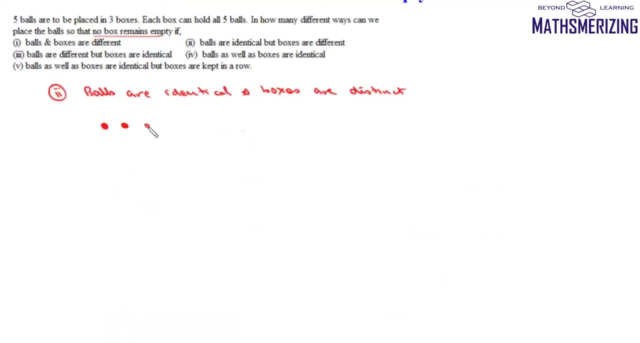 So here we have five balls which are identical, But in this case they are not identical. boxes are distinct. so we have five identical balls and three distinct boxes. now in how many ways we can distribute these identical balls in these boxes? so in the first question we have discussed 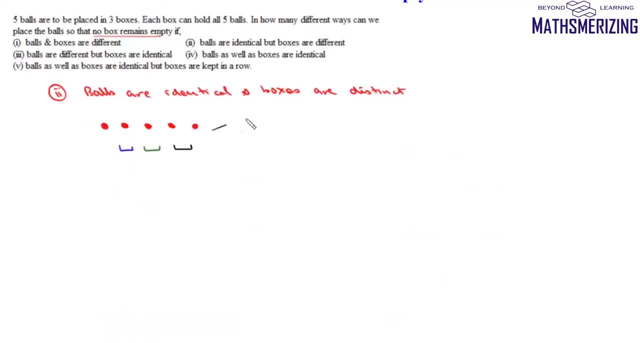 how to distribute these identical balls in identical boxes. so it can be done in two ways: either we can distribute them as 2, 2, 1, or we can distribute them as 3, 1, 1. now, once we have distributed these balls as 2, 2 and 1, now, since these three boxes, they are distinct, so it matters. 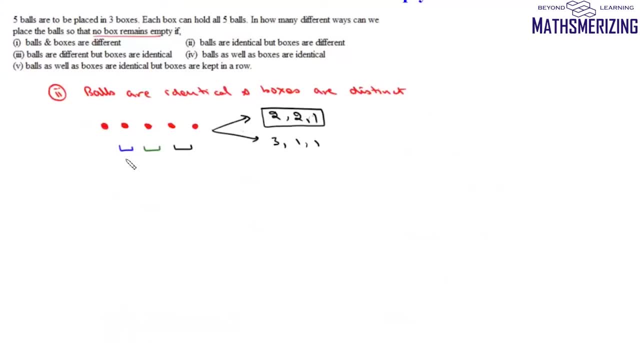 which box has this one ball? it could be either 2 in blue, 2 in green and 1 in black, or it could be 1 in green or it could be 1 in blue, so we can distribute 2, 2 and 1 in three distinct boxes, as 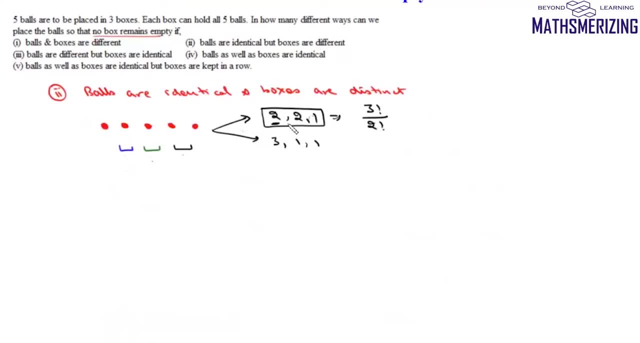 factorial 3 divided by factorial two ways, because here these two numbers, they are same. so it can be done in only three ways and we know that it will be either you 2, 2, 1 or 2 1, 2 or 1 2, 2. in the same way, we can distribute 3, 1, 1 in 3 distinct boxes, as 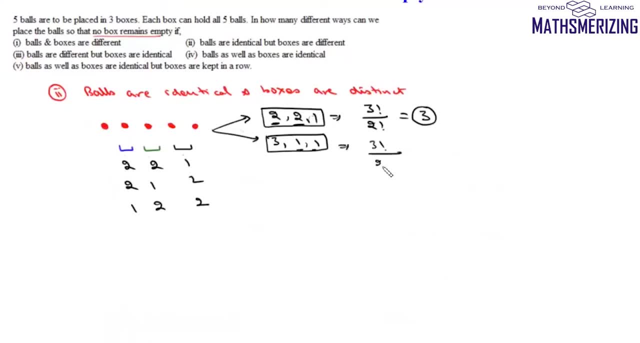 factorial 3, and then again we have 2: 1 same, so it will be divided by factorial 2, and this again is 3, so it will be 3 plus 3, and that is 6 ways. so we can write this as 3, 1, 1, 1, 3, 1 or 1: 1, 3. 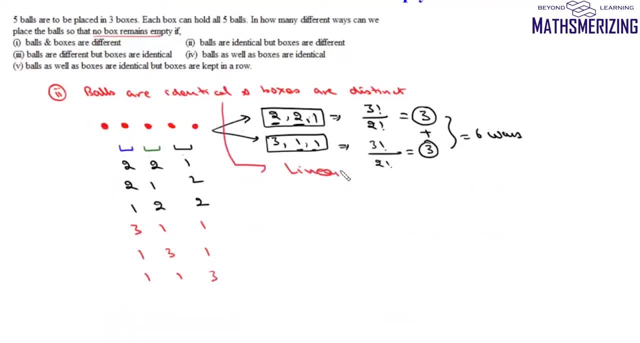 now, the best way to solve such questions is using linear equations. so what we'll say is we'll say: let number of balls in first box be x1, let the number of balls in second box be x2 and number of balls in third box be 3. 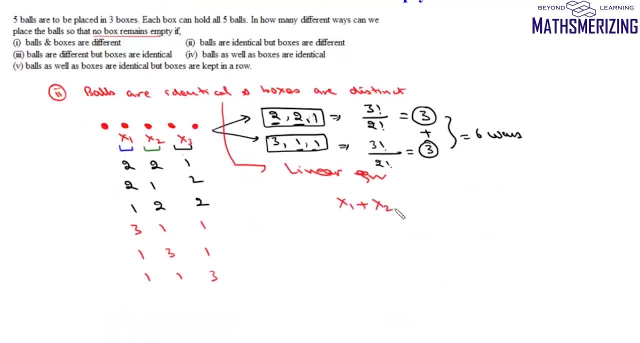 then we can simply write this equation as: x1 plus x2 plus x3, and it is equal to n, so which is equal to number of balls in this case. so once we have identical objects and we have to distribute these identical objects into distinct groups, then we can always use this linear equation. 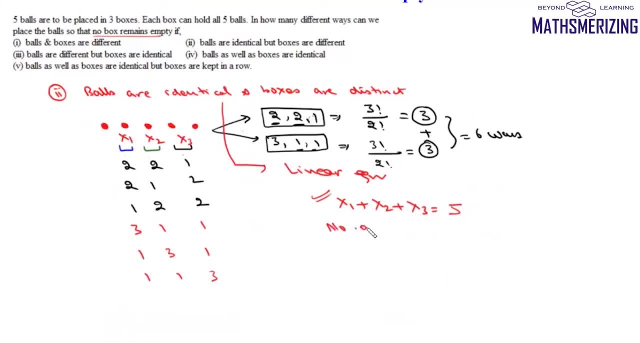 so here we need to find number of positive integral solutions. so we know that number of positive integral solution is given by n minus 1, which is 5 minus 1 c, r minus 1. r in this case is 3, so it will be 3 minus 1, so that should be 4 c2, and 4 c2 is nothing but 6. 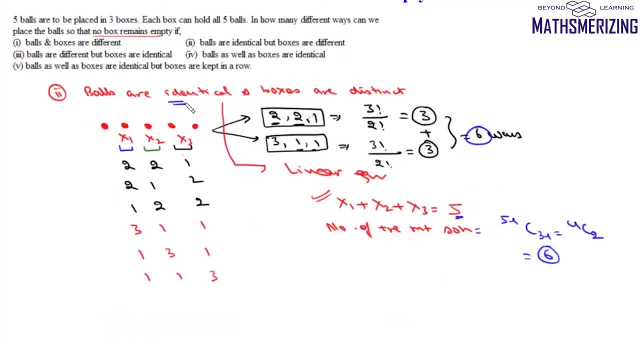 so total number of ways in which we can distribute identical balls into distinct boxes is 6. now if we have general questions- say we have n identical balls and r distinct boxes, then we can simply write this equation as x1 plus x2 plus xr, one for each box, and it should be equal to n, and number of positive integral solution is given by n minus 1, c, r minus 1. so this is how we can find the cases when the balls are identical and boxes are distinct and each box should have at least one ball. now we'll come to this. 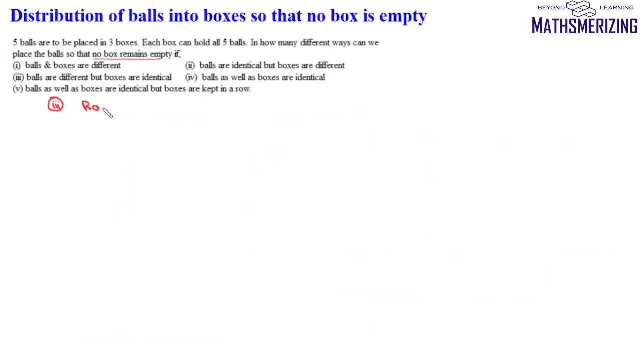 third case, when 3 Balls are distinct but boxes are identical. So here, in this case, we have distinct balls but identical boxes. So we have five distinct balls, So one, two, three, four and five. So we have five distinct balls and three identical boxes. 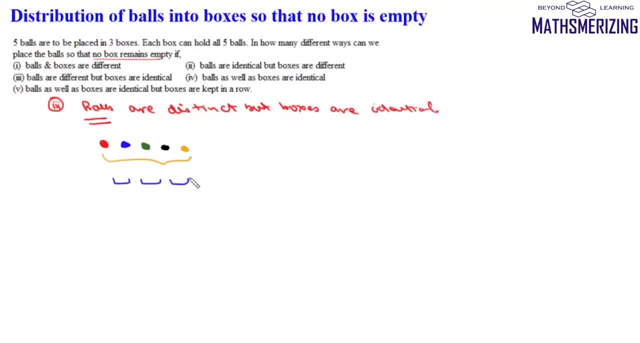 So now we need to distribute distinct objects in identical cases. Now in this question we already know that we can distribute five balls in three boxes, so that no box is empty, In either two, two or one way, or we can distribute them as three, one or one way. 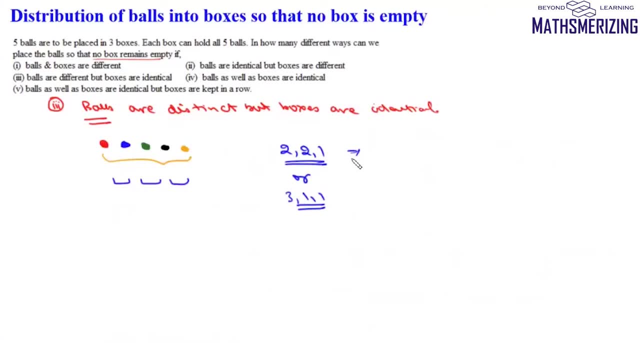 Now, this question is actually nothing, but it is distribution of objects into identical groups. Now, how do we distribute five objects in a group of two, two and one? So we know that this can be done in factorial five divided by factorial two. factorial two. 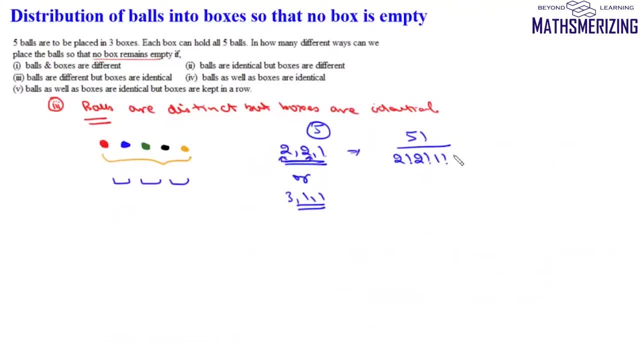 factorial one, And since we have these two numbers same, we need to divide it with factorial two. So it will be Okay: One twenty divided by eight, So it will be fifteen. Now, in the same way, we need to distribute five objects in a group of three: one one. 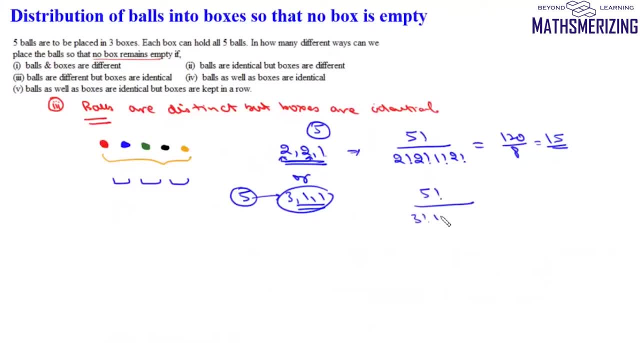 So it will be factorial five, factorial three, factorial one, factorial one, And since these two they are identical, we again need to divide it with factorial two. So it will be again one twenty, and here it is six into two, So which is ten. 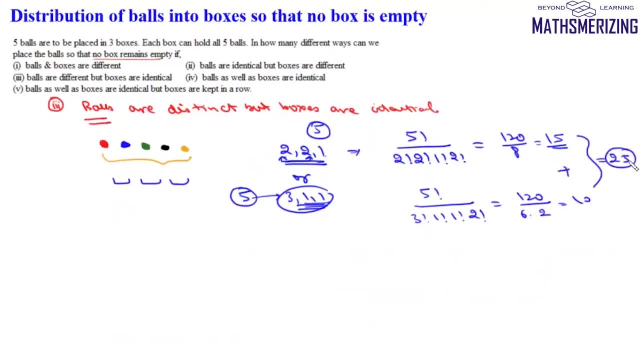 So it will be simply fifteen plus ten, and that should be twenty five. So number of ways of distributing Five distinct balls in three identical boxes is twenty five. So this problem is actually distribution problem, which we generally study in combinations: distribution into non distinct groups. 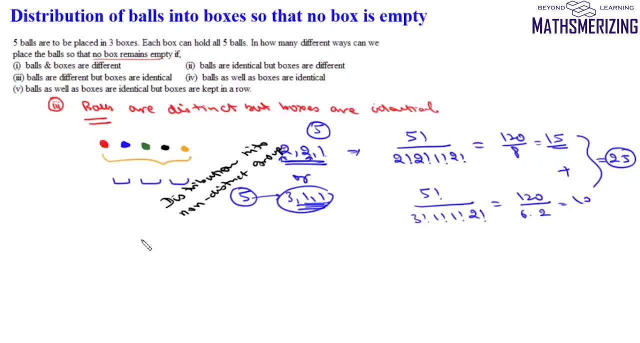 Now let us discuss more general problem. in this Suppose we have n distinct balls And are identical boxes. So you know how many ways we can distribute n distinct balls in our identical boxes so that no box is empty. Now it can be done in S and R ways. 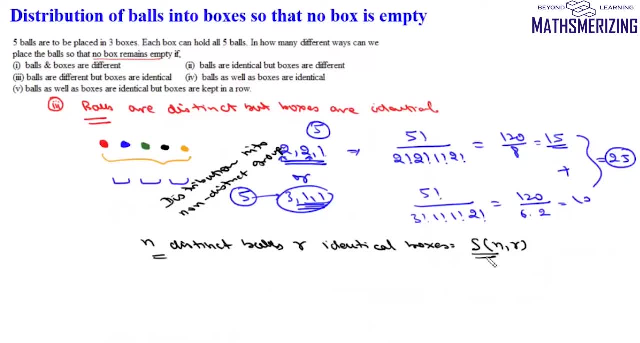 So there is a direct formula for this: S and R. and S and R is nothing, but it is a sterling number of the second kind. Now how do we find S and R? So this is a formula for S and R. S and R is given by: 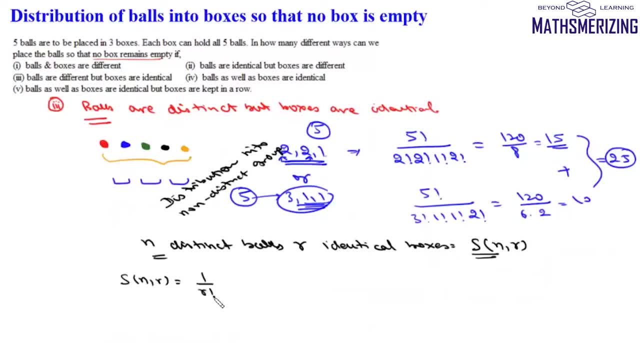 One upon factorial R, and then it will be R C zero. R to the power n minus R C one. R minus one to the power n, plus R C two. R minus two to the power n. And you continue till the end where it will be minus one to the power R minus one one. 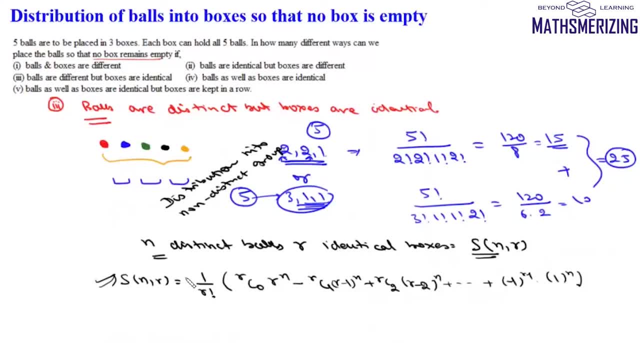 to the power n. So using this formula, we can find out this Sterling number, SNR, and this SNR is equal to number of ways in which we can distribute n distinct balls in r identical boxes. So we'll use this formula for r question and this value of n is 5 and value of r is 3.. So we need to find. 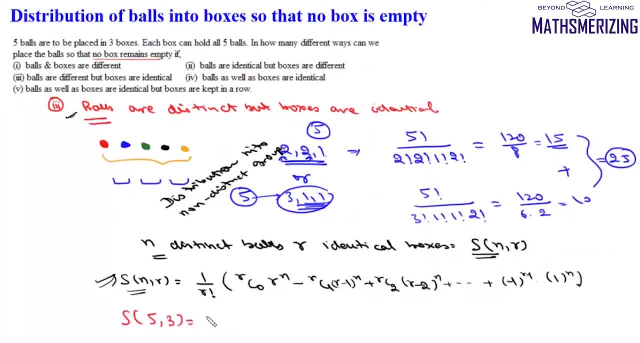 S53.. Now S53 will be 1 upon factorial 3, 3C0,, 3 to the power 5 minus 3C1,, 2 to the power 5 plus 3C2, 1 to the power 5.. So we need to find this number and this number is S53.. Now this is 1. 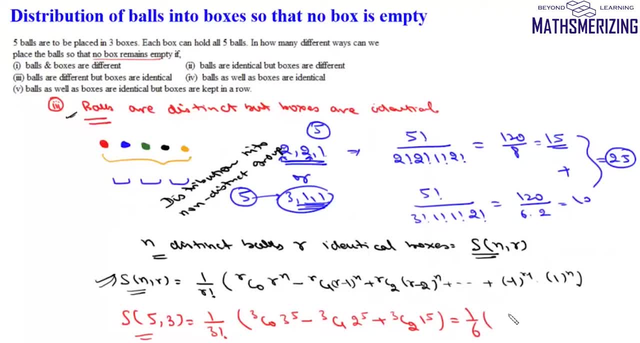 upon factorial 3, which is 6.. Now 3 to the power 5, 3 to the power 5, 3 to the power 5, is 243. minus 2 to the power 5, it is 32.. 32 into 3 is 96. And then plus 3C2, it is simply 3.. So 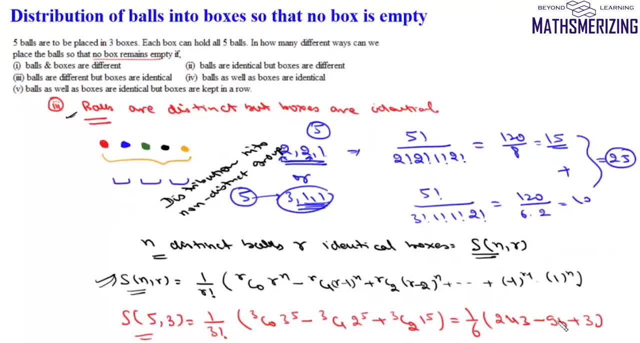 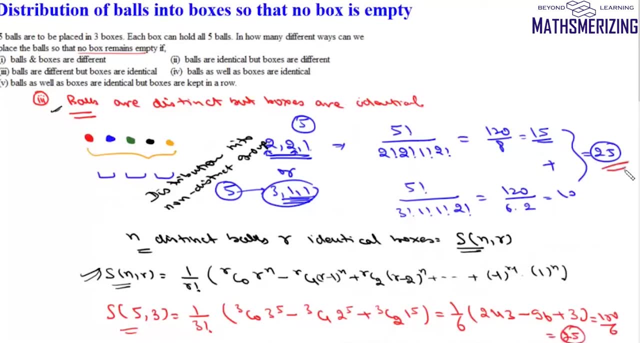 we'll get 246 minus 96.. So it'll be 150.. And 150 divided by 6 is simply 25.. So which is the answer to r question? So a general way of solving this question is by finding this Sterling number, SNR. 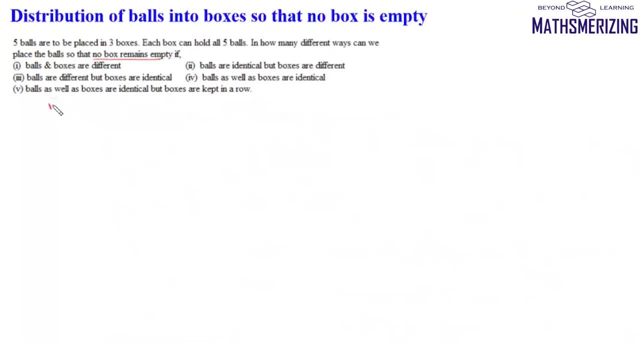 is equal to number of ways in which we can distribute n distinct balls in r identical boxes Using this given formula. Now we'll come to our fourth case, which is when the balls are distinct and boxes are distinct. So now we have five balls. 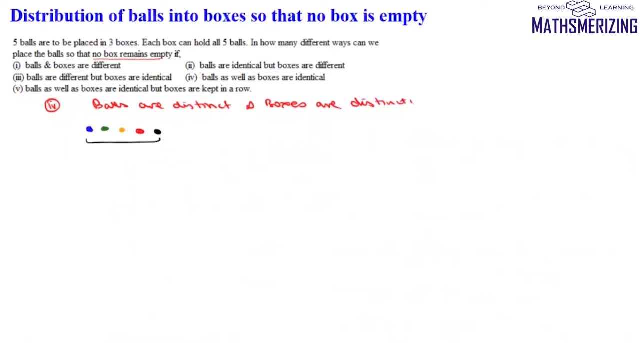 Which are distinct, And we also have three boxes which are distinct. Now, with distinct balls and distinct boxes, we need to distribute the balls so that no box is empty. So in the previous case we have studied that when the balls and boxes are identical, we can distribute them as 3, 1, 1, and then 2,, 2 and 1.. So what we'll do is we'll 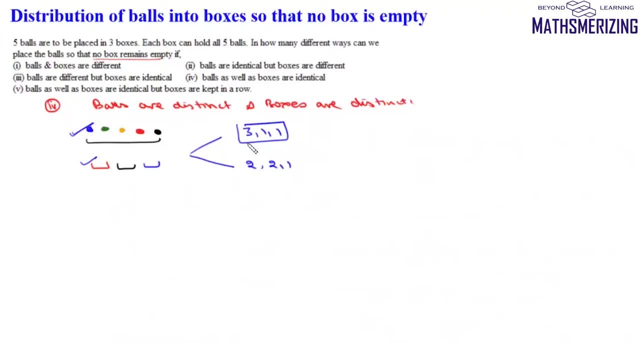 first distribute these five balls in a group of three, one and one, and then we'll arrange this three, one, one in these three boxes. so first we'll go for distribution. distribution part will be factorial five divided by factorial three, factorial one, factorial one, and then these ones are same. so 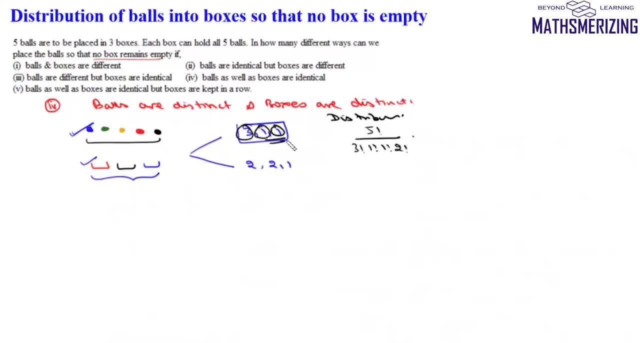 it'll be divided by factorial two, and then now we have three objects and these three objects are to be arranged in these three boxes. it can be done in factorial three ways. so now it will be 10 into 6, that is 60 and the same way. first we are going to distribute two, two and one, so it'll be factorial. 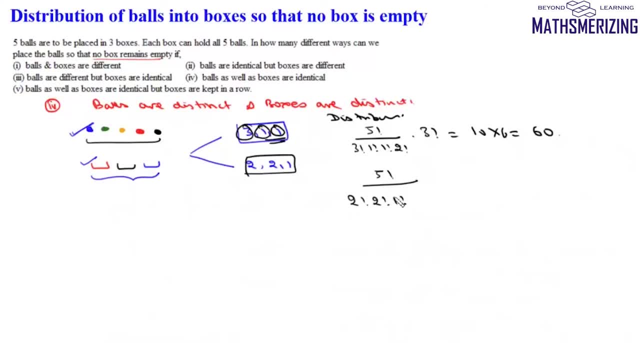 five, factorial two, factorial two, factorial one, and then again these two and two. they are same, so it'll be factorial two and again we have three objects and they are to be arranged in three places. it can be done in factorial three ways, so here it will be 15 into 6, that should be 90. so total number of ways of distributing five distinct balls. 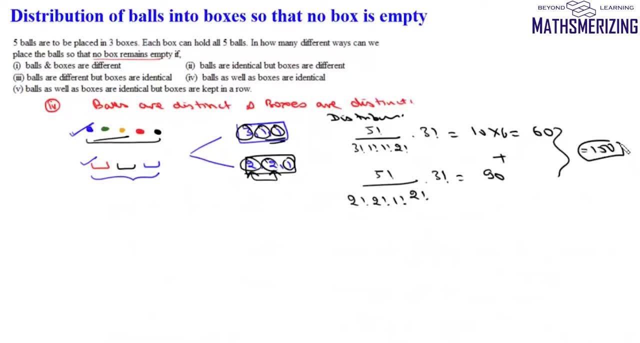 in three distinct boxes is 150. now what is the general way of solving this problem? generally, we are solving this problem. then we have n distinct balls and they are to be distributed in our distinct boxes such that no box is empty. now this problem is given by 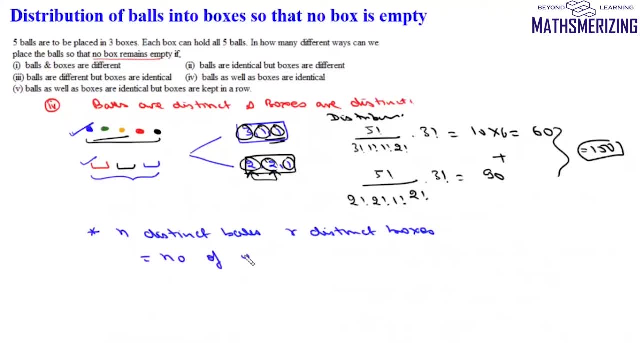 number of onto functions, from a set containing n elements to set containing r elements. we have already done a video on number of onto functions, so i'll provide the link to that video in the description below for your kind per user, so you can have a look at that video to find out how we 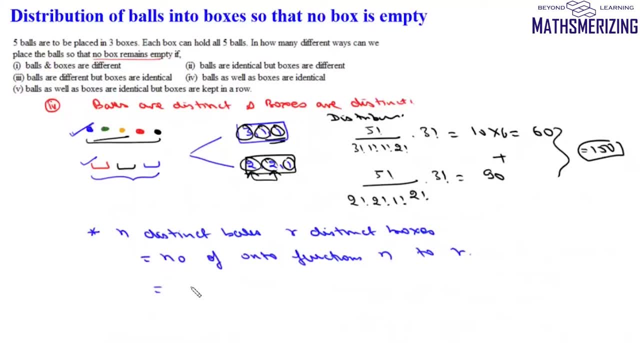 have worked out a formula. number of onto functions is given by r to the power n minus, and then r- c1. r minus one to the power n minus, Rc2. r minus two to the power n and we continue up to minus one to the bar, r minus one and then. 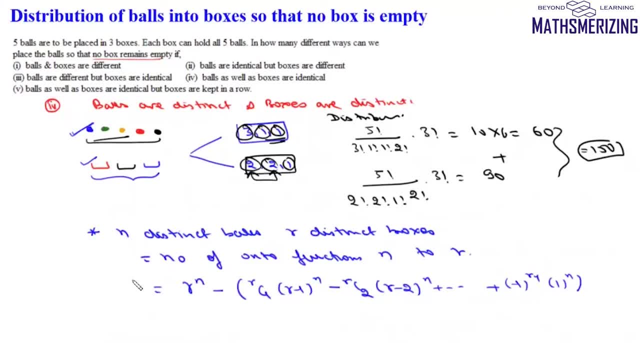 1 to the power n. so this is the formula for number of onto functions from n to r. so in our case the value of n is 5 and the value of r is 3, so total number of ways of this distribution will be r to. 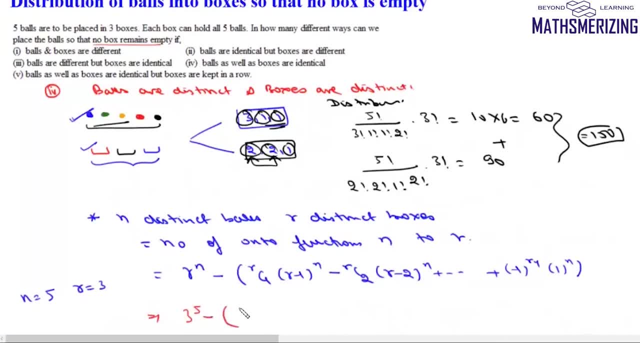 the power n, so will be 3 to the power 5 minus 3 c 1. 2 to the power 5 minus 3 c 2. 1 to the power 5, so 3 to the power 5, it is 243 minus 3 c 1 is 3, and 2 to the power 5 is 32 and minus 3, so there. 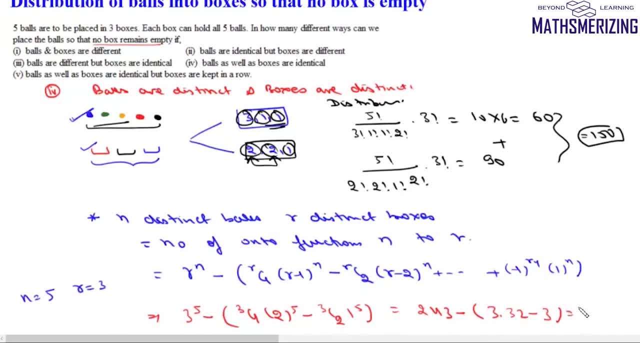 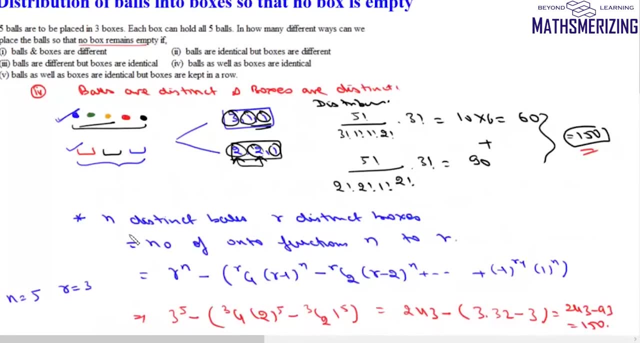 will be 96. 96 minus 3 is 93, so it will be 243 minus 93, which is nothing but 150. so this is how we can find number of ways in which we can distribute n distinct balls in r distinct boxes. now coming to this fifth case,